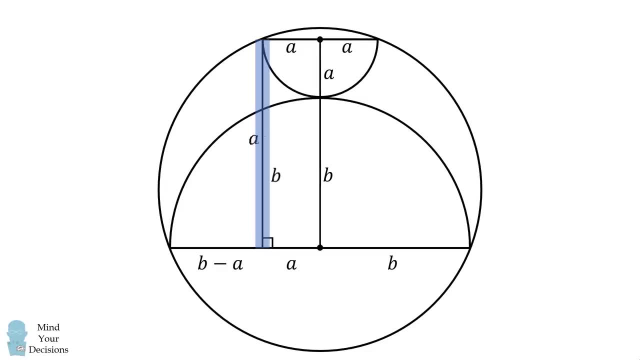 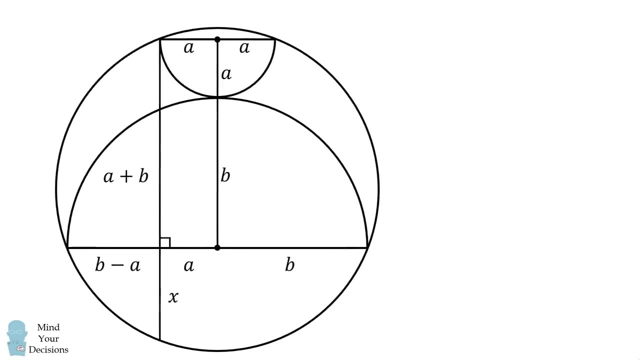 The other side of the rectangle will have a length equal to a plus b. From here we will extend this side of the rectangle to be a chord of the large circle. Suppose the length here is equal to x. We can solve for the value of x by the intersecting chords theorem. 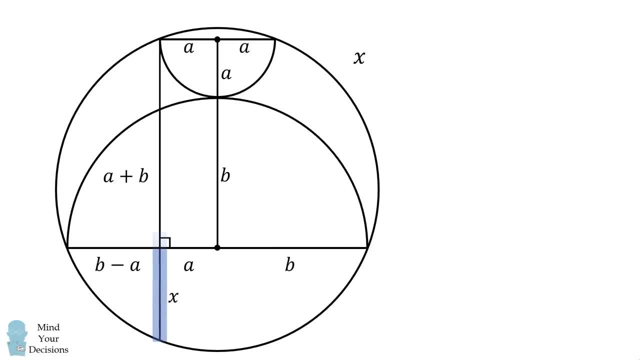 We have: x multiplied by a plus b is equal to b minus a. multiplied by a plus b, We'll solve for x and we'll cancel out the term a plus b in the numerator and the denominator. Thus x is equal to b minus a. 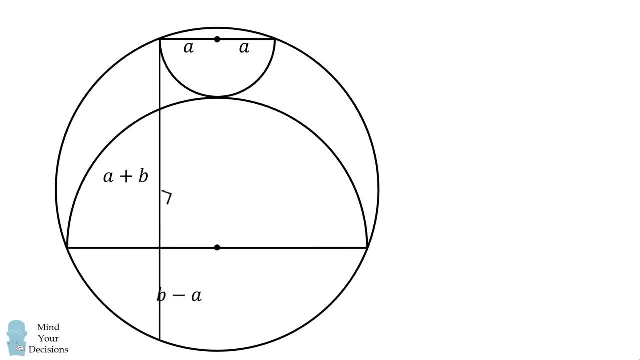 We then will simplify this diagram and we'll consider the following right triangle- Notice- we have an inscribed angle that's equal to 90 degrees. Therefore, the chord opposite this 90 degree inscribed angle, will be a diameter of the circle. 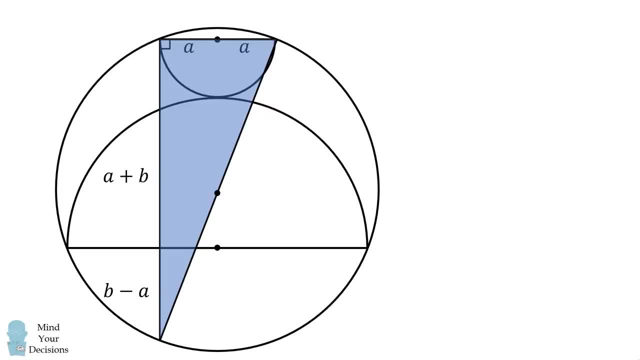 In other words, this chord passes through the center of the circle and its length will be equal to 2 times the radius of the circle. We can then use my favorite right triangle theorem. We will have the square of 2a plus the square of 2b is equal to the square of 2r. 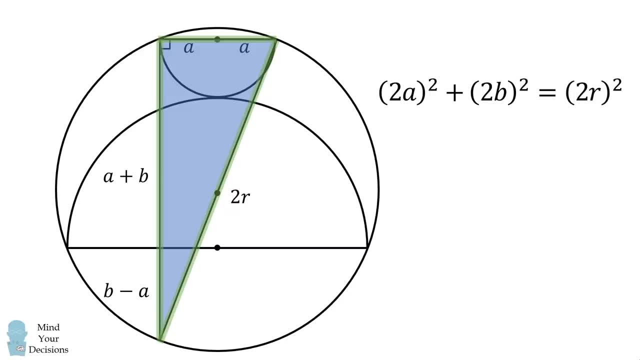 We can square each of these terms and then simplify by dividing both sides by 4 to get a squared plus b squared is equal to r squared. From here we can solve the problem. The area of the large circle is equal to 1, which means pi r squared is equal to 1.. 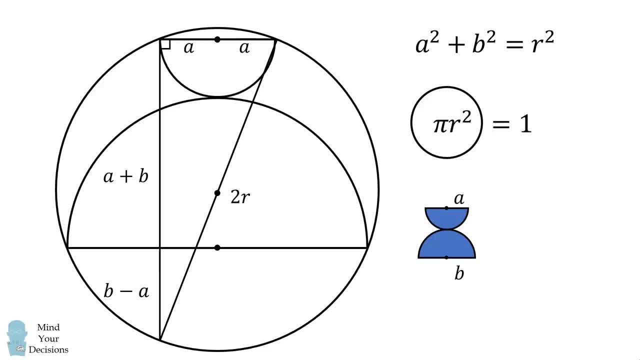 We can then calculate the combined area of the two semicircles. It'll be equal to 1 half pi multiplied by a squared, plus 1 half multiplied by pi multiplied by b squared. We can then simplify this and we can then substitute that a squared plus b squared is equal to r squared. 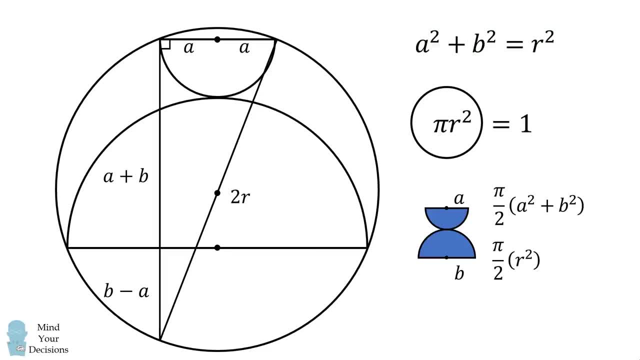 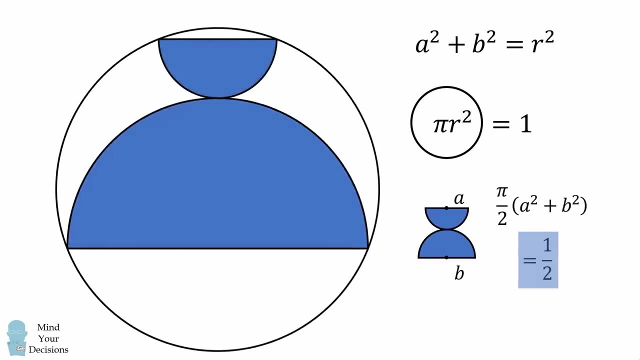 We thus have pi over 2 multiplied by r squared, But we know that pi r squared is equal to 1.. Therefore, pi over 2 multiplied by r squared must be equal to 1 half, And that's the answer. It's rather remarkable that the combined area of the two semicircles 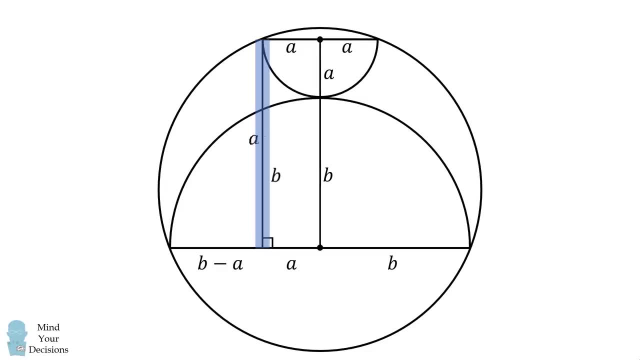 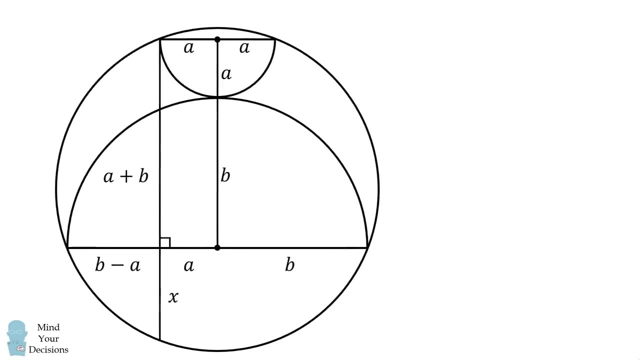 The other side of the rectangle will have a length equal to a plus b. From here we will extend this side of the rectangle to be a chord of the large circle. Suppose the length here is equal to x. We can solve for the value of x by the intersecting chords theorem. 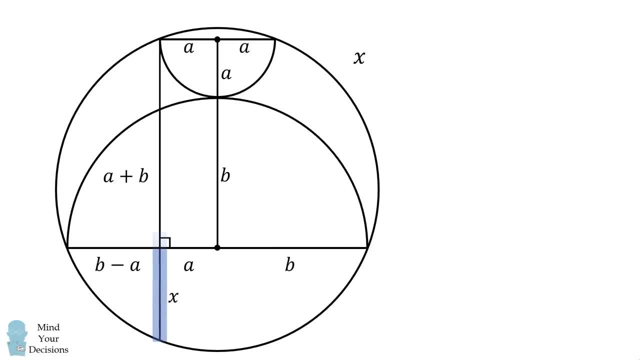 We have: x multiplied by a plus b is equal to b minus a. multiplied by a plus b, We'll solve for x and we'll cancel out the term a plus b in the numerator and the denominator. Thus x is equal to b minus a. 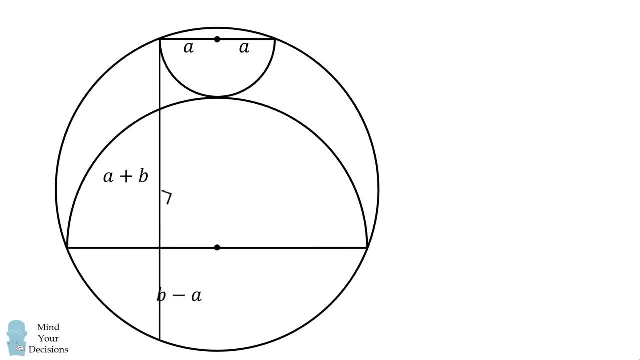 We then will simplify this diagram and we'll consider the following right triangle- Notice- we have an inscribed angle that's equal to 90 degrees. Therefore, the chord opposite this 90 degree inscribed angle, will be a diameter of the circle. 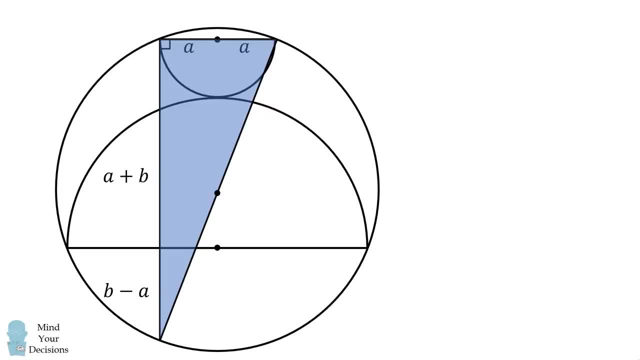 In other words, this chord passes through the center of the circle and its length will be equal to 2 times the radius of the circle. We can then use my favorite right triangle theorem. We will have the square of 2a plus the square of 2b is equal to the square of 2r. 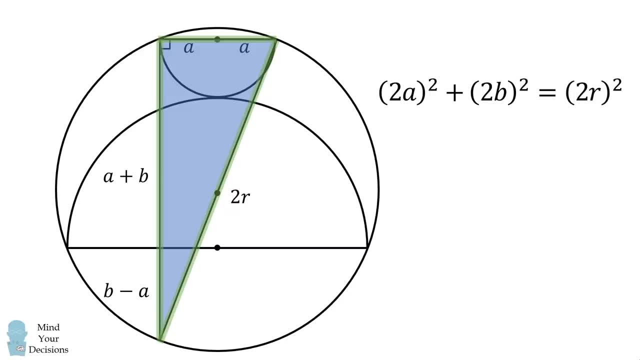 We can square each of these terms and then simplify by dividing both sides by 4 to get a squared plus b squared is equal to r squared. From here we can solve the problem. The area of the large circle is equal to 1, which means pi r squared is equal to 1.. 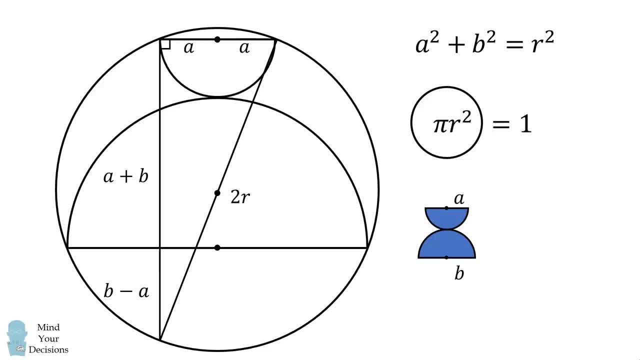 We can then calculate the combined area of the two semicircles. It'll be equal to 1 half pi multiplied by a squared, plus 1 half multiplied by pi multiplied by b squared. We can then simplify this and we can then substitute that a squared plus b squared is equal to r squared. 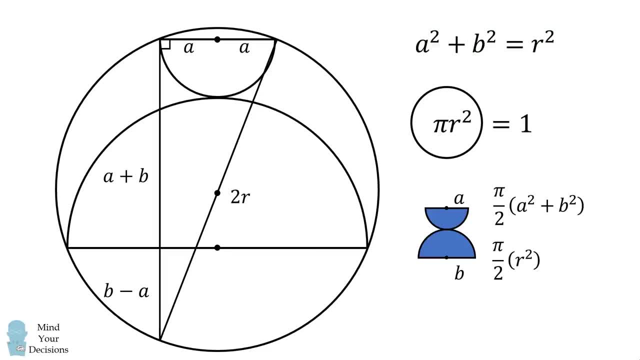 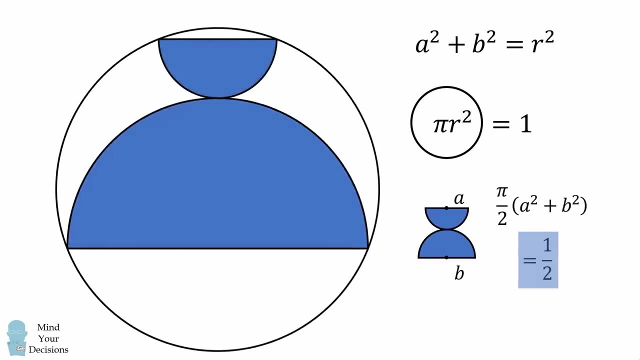 We thus have pi over 2 multiplied by r squared, But we know that pi r squared is equal to 1.. Therefore, pi over 2 multiplied by r squared must be equal to 1 half, And that's the answer. It's rather remarkable that the combined area of the two semicircles